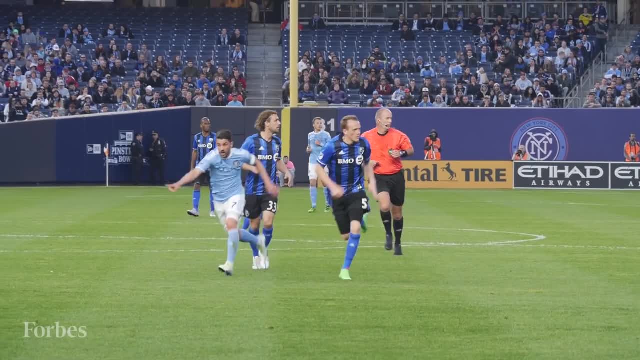 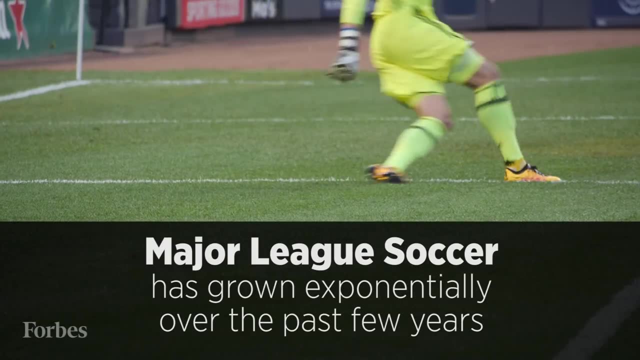 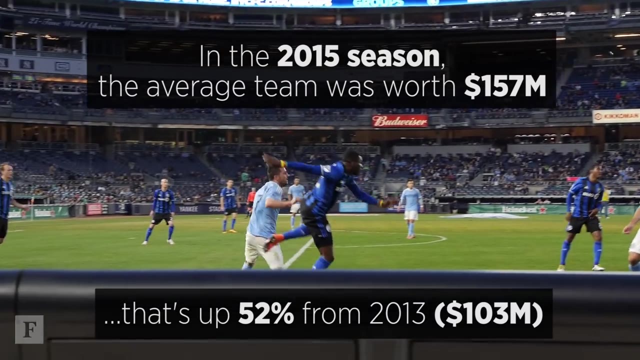 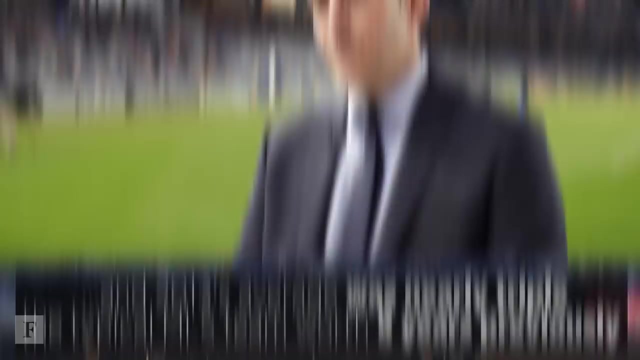 The best leagues in the world have 100 years. It needs time, it needs a lot of work, but we are in the road for it to be one of the best leagues in the world. We all know that soccer is on an incredible growth trajectory on a global level. 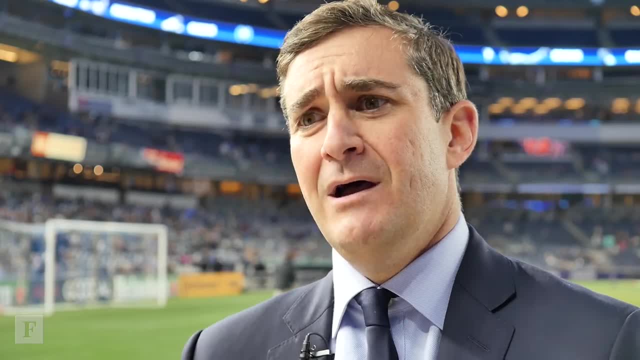 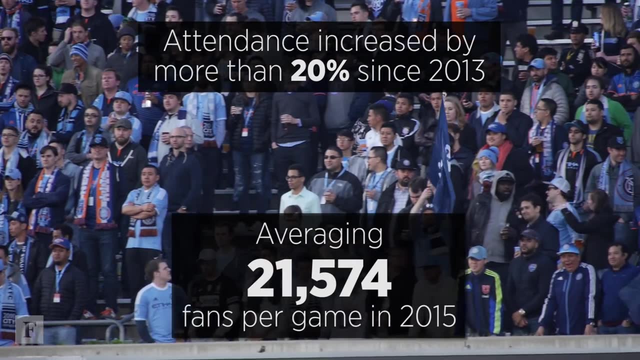 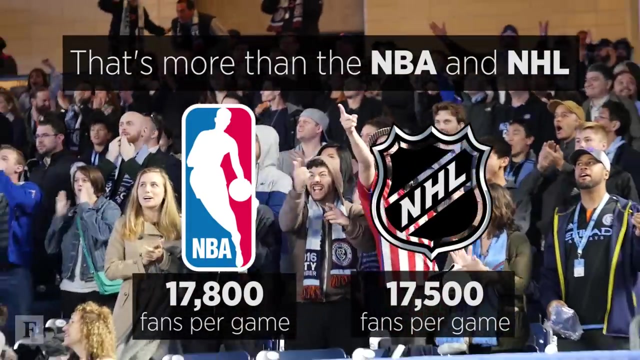 and here in the US as well, and especially here in New York. Attendance is up, the TV ratings are up and we're seeing interest at all levels. I went to a Rapids game when I was 12 or 13 years old. 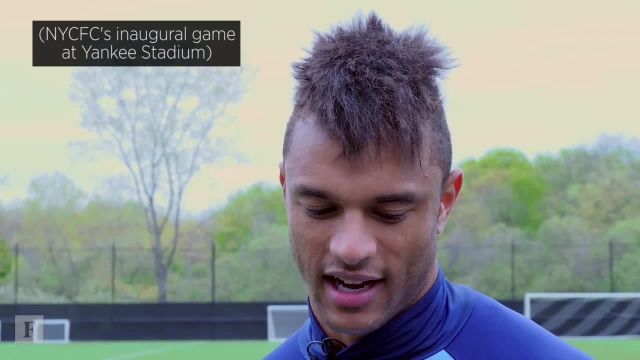 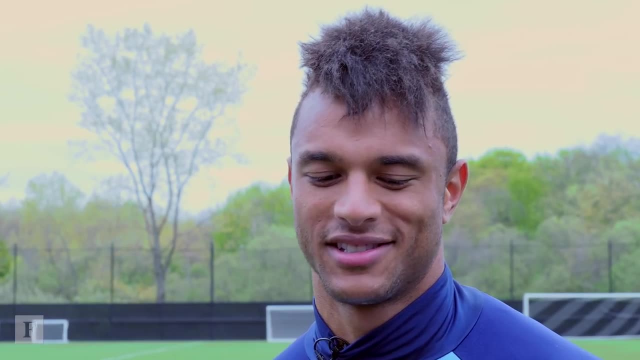 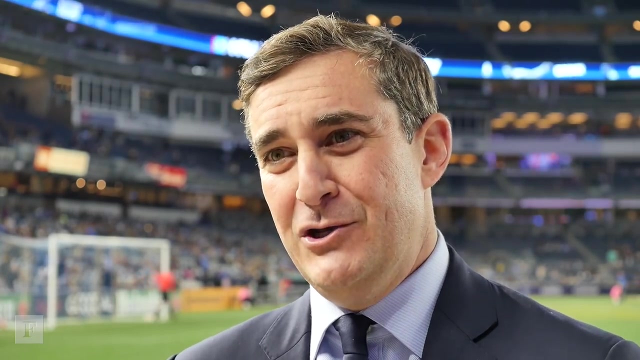 Not many fans were there the first game. I can't explain the feelings I had. The fans were loud cheering my name. It was amazing, As the MLS is an up-and-coming league. we are younger. It's always fun to be the newer, upstart and be more entrepreneurial. 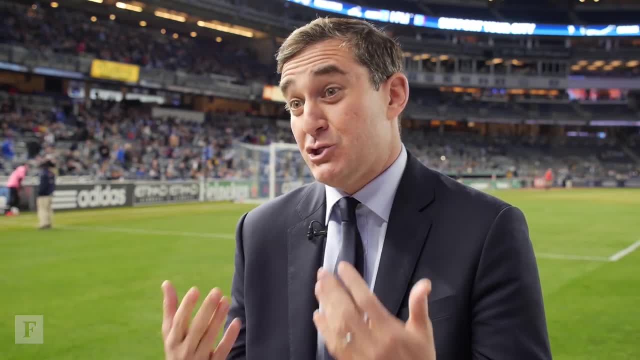 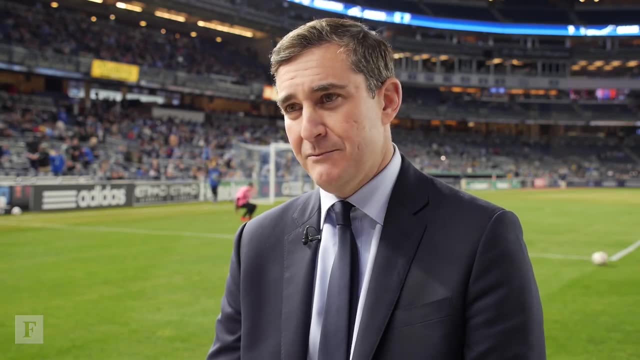 We talk a lot about being a club that's disruptive. I like that idea of us taking the norms, taking what's been done before and challenging it a little bit, looking at problems in different ways and really trying to push the envelope. 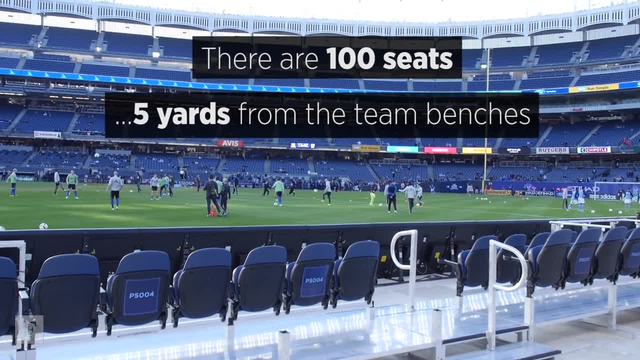 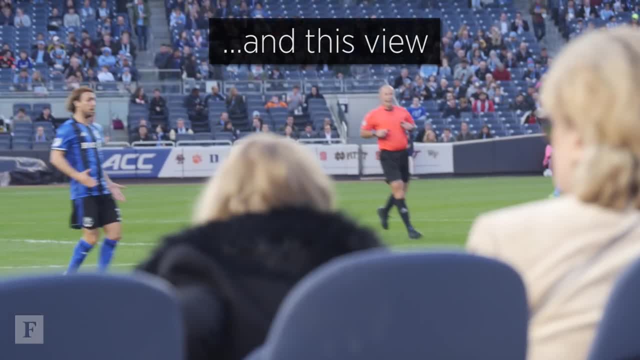 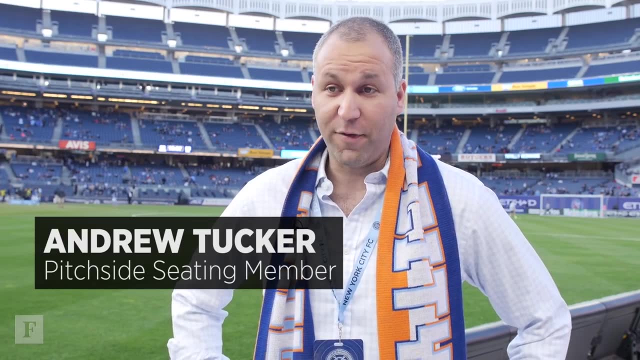 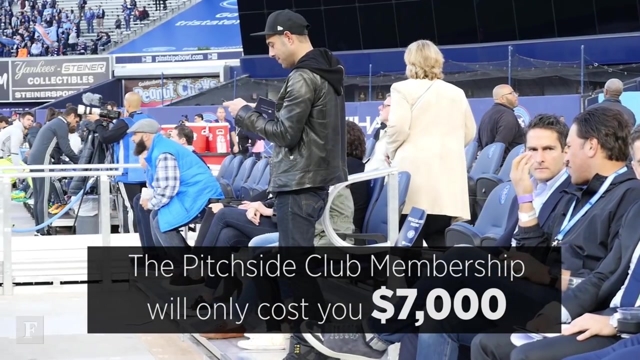 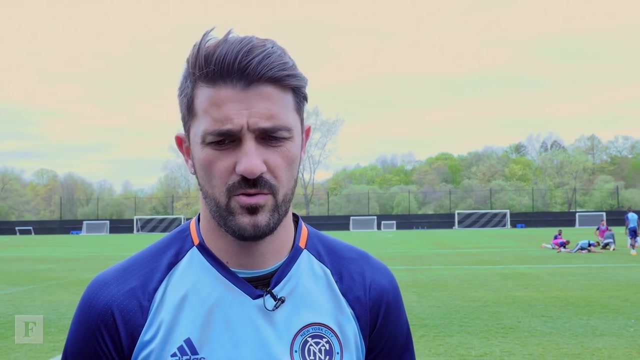 Soccer players get a pretty bad rap for acting and faking injuries, but when you're this close to the action, you see the impact of those tackles. It's very good for us to have our fans too close and it's very interesting for the fans. 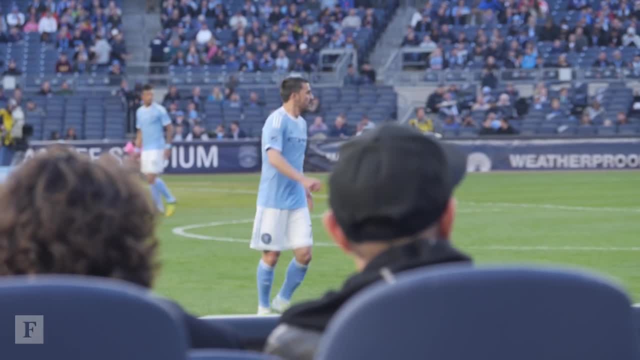 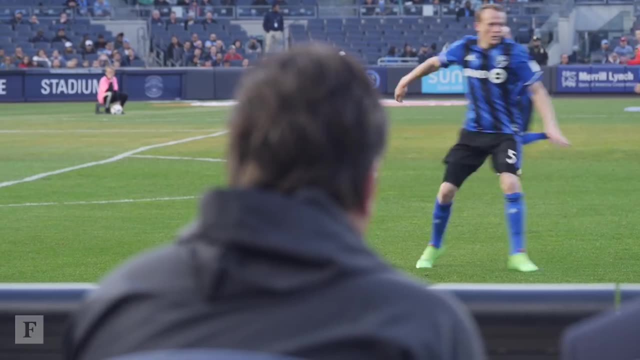 to have the opportunity to stay close to the players, close to the pitch, close to the field. It's nice knowing that we have fans right next to us so we don't feel kind of spaced out from them. I think it's. I think they also enjoy them.